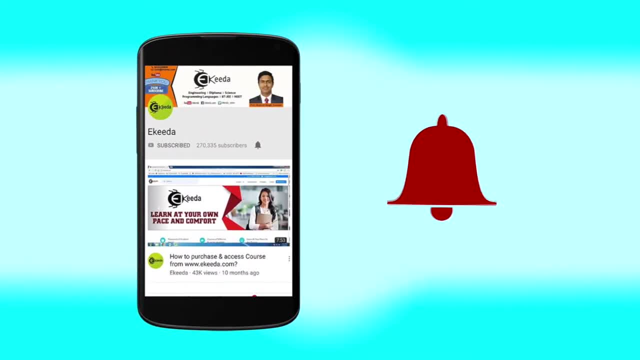 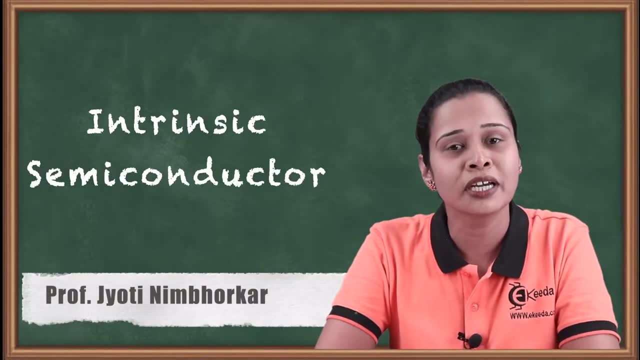 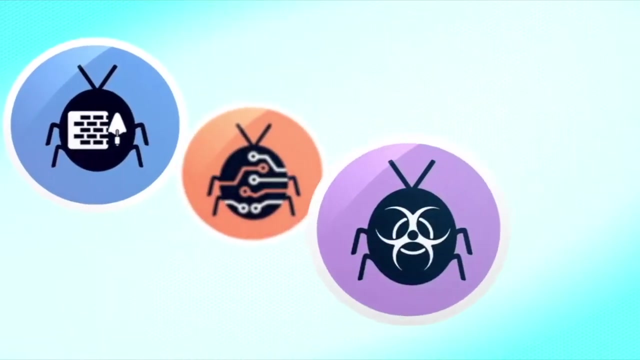 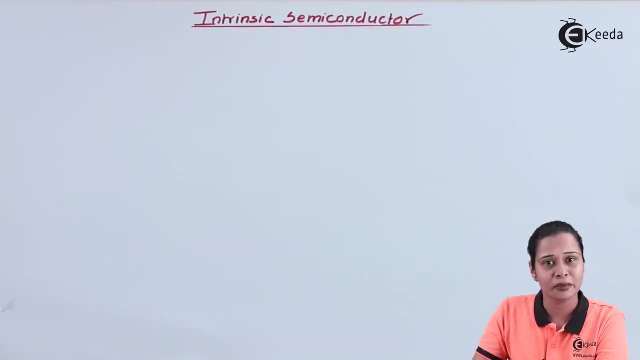 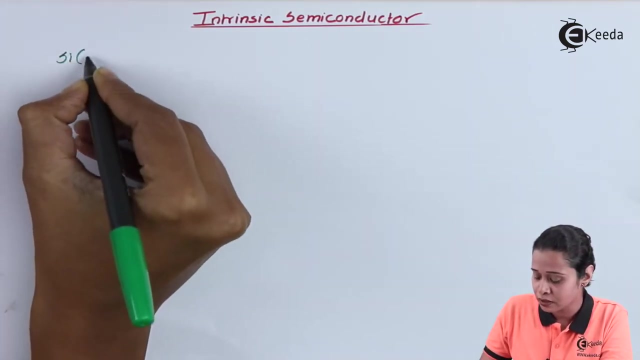 Click the bell icon to get latest videos from eKIDA. So let us see briefly what is intrinsic semiconductor. Now let us start with intrinsic semiconductor. We will take example of silicon. We know in silicon configuration is 2,, 8 and 4.. So there is a configuration of 2, 8 and 4. So there are 4 valence electron For completion of octet. that silicon required 4 more valence electron, So this silicon making covalent bond with other silicon atom. 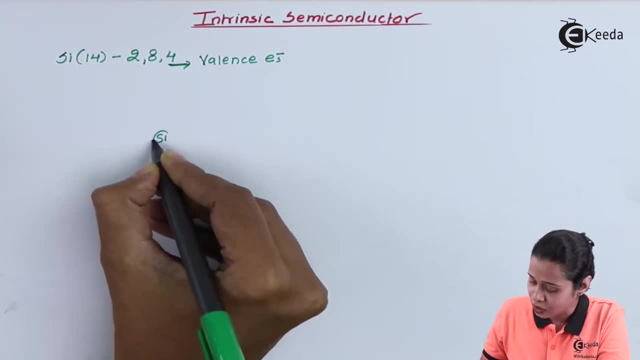 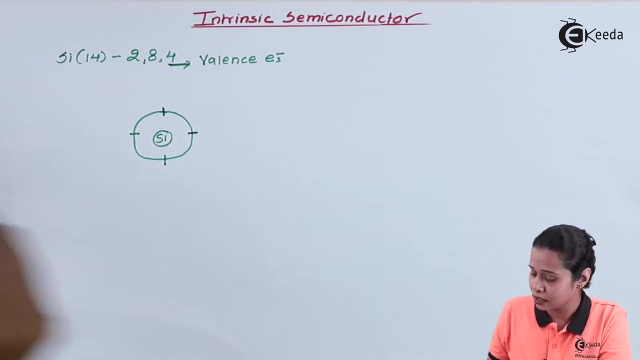 So let us see, Consider: this is the first silicon atom and it has 4 valence electron. We will only draw the outermost orbit. So here it has 1 electron, the second one, third and fourth. Now this silicon atom making covalent bonding. 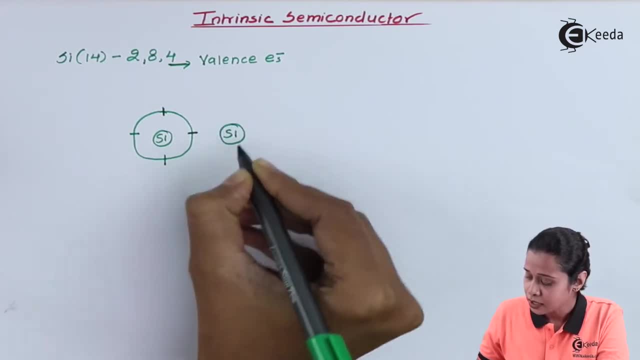 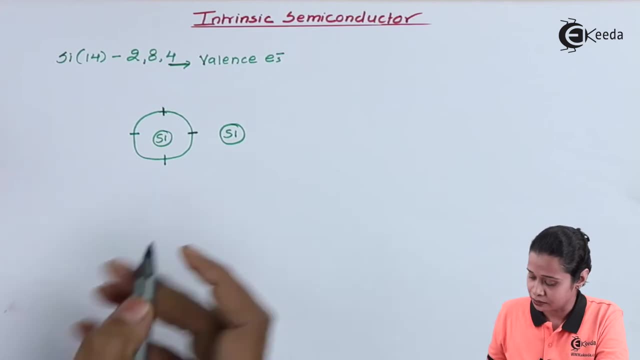 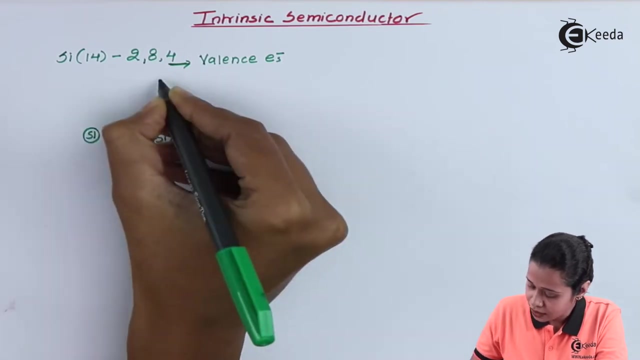 with another silicon atom, because this silicon atom is also having 4 valence electron. So let us consider 4 neighboring silicon atom. So this is the first one We have here, second silicon, third silicon and here we have a fourth silicon atom. 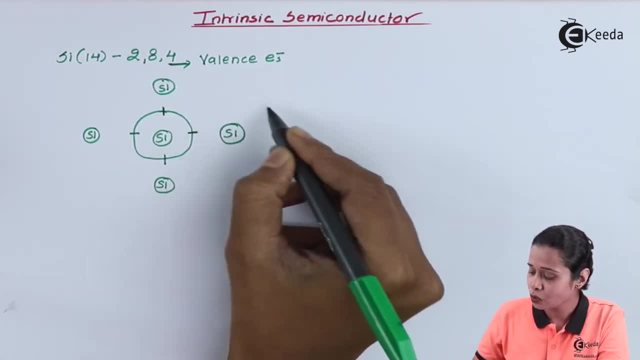 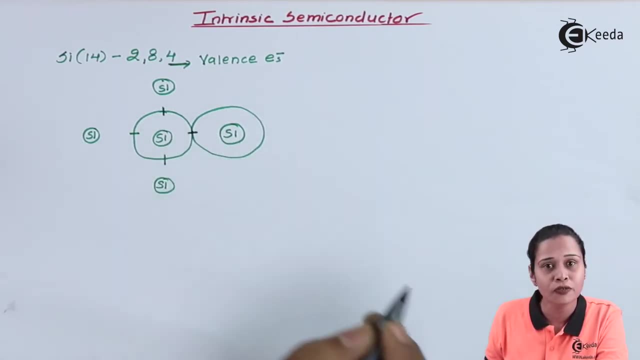 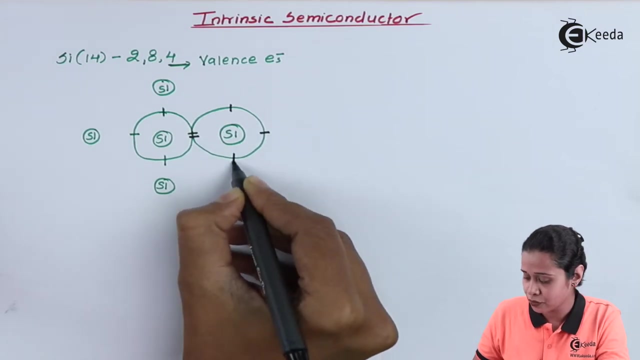 Now consider: this is the outermost orbit of this silicon like this, and this outermost orbit is also having 4 valence electron. So let us see, This is the first one, second, third and fourth. We have another silicon neighboring atom. This is the valence shell of the. 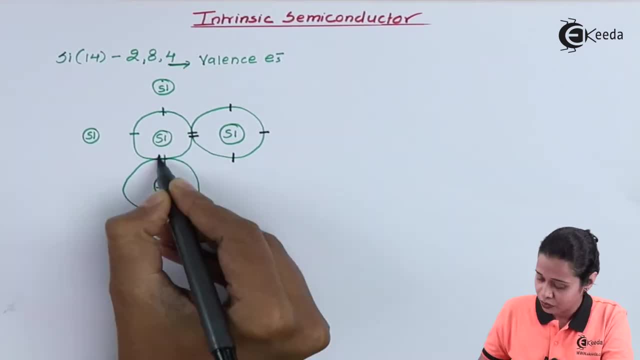 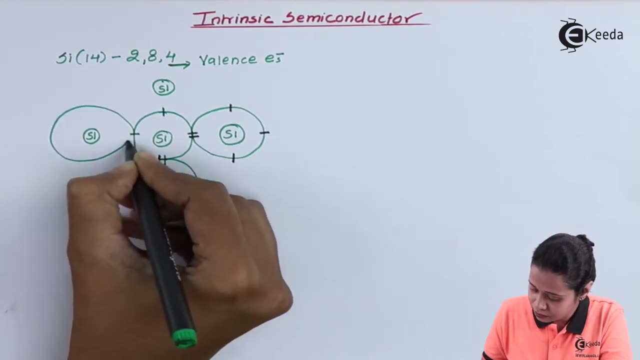 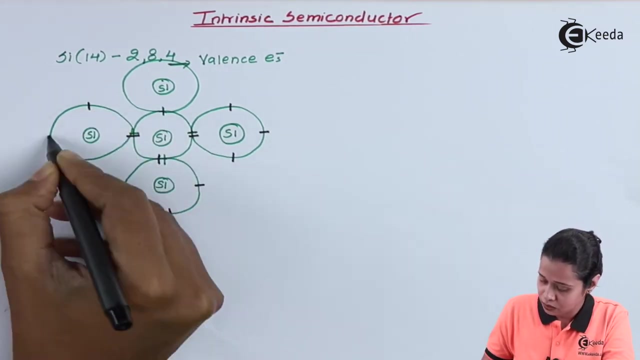 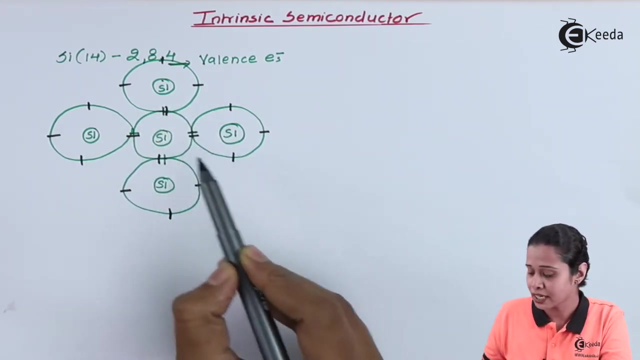 second neighboring silicon. Again, it has 4 valence electron. We will consider third one and fourth one. So in this way we have Now, when we look at the central silicon atom, that central silicon having 8 electron in its 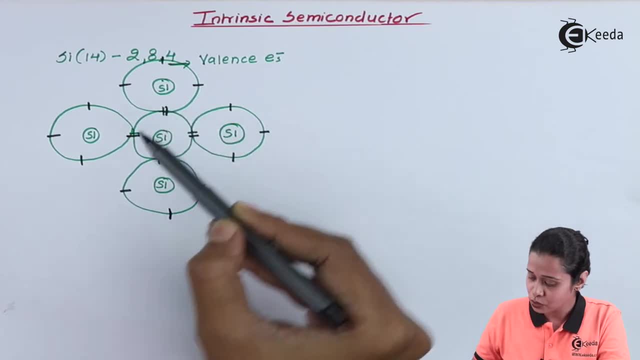 outermost shell, This 2 electron, this 2, 2 and 2.. So there are total 8 electron in the outermost orbit. So this is the outermost orbit of this silicon. So let us consider third, one and fourth one. 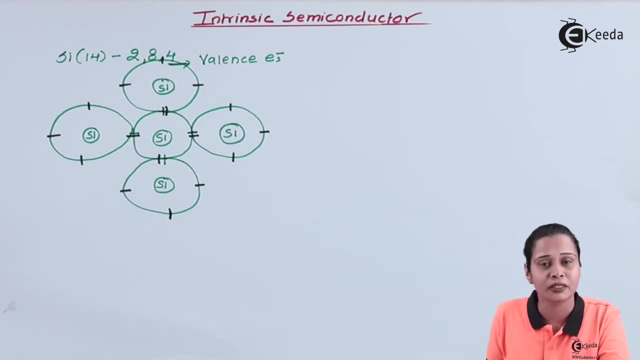 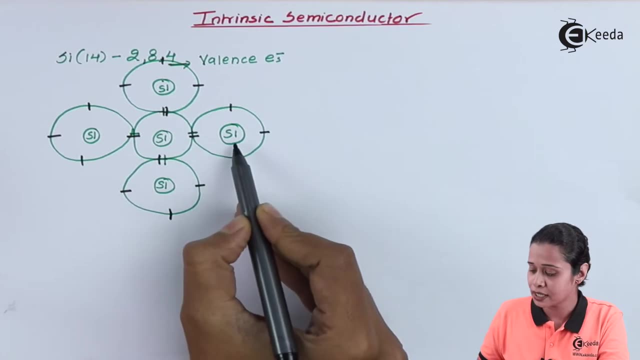 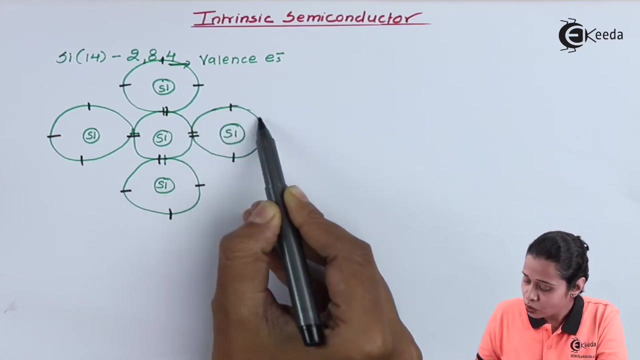 Means that central silicon is a stable one, That is, its octade is complete. Now this silicon will move. For example, we are considering this silicon atom. Then the electron of this silicon atom will move to its own orbit like this, in this way: 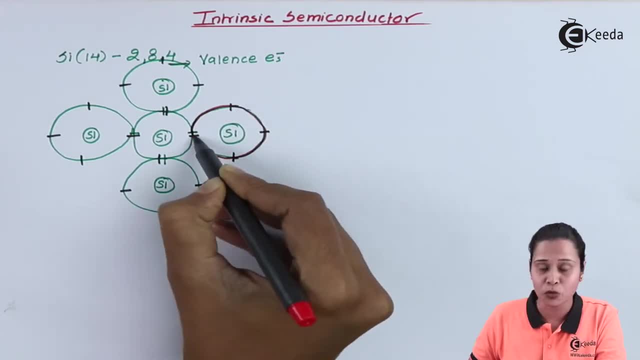 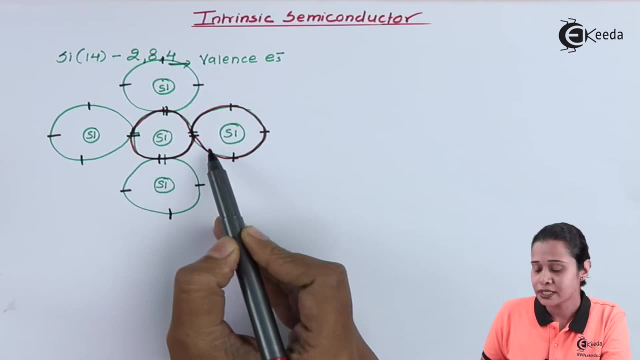 and then it will move around the another silicon atom like this. In this way the silicon of this atom will take one complete round around both the silicon. So this type of bonding is called as a covalent bonding. Similarly we can say the valence. 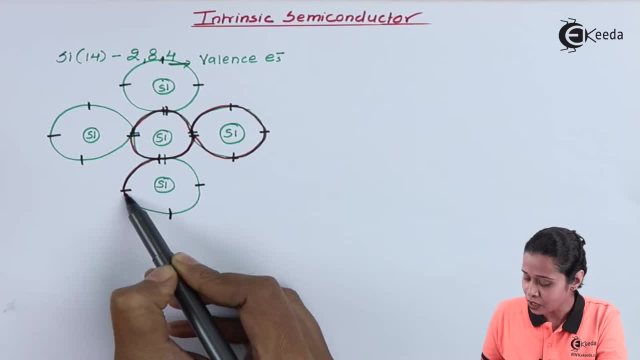 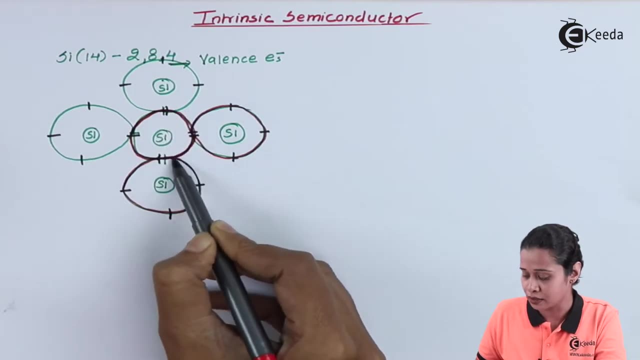 electron of this silicon will again take one round around its own atom and then the second round of the shared silicon atom in this way, So we can say there is such a covalent bonding in silicon solid for the stable structure. If you want to draw it more properly, then we will go. 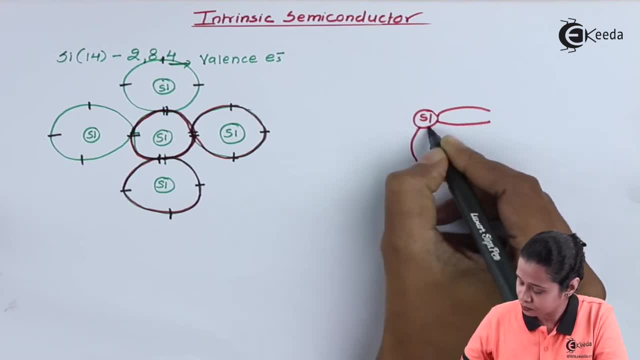 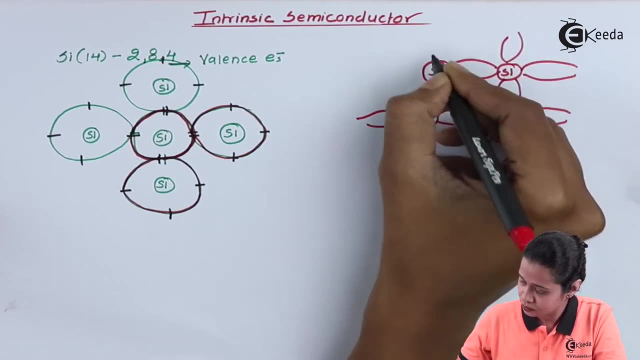 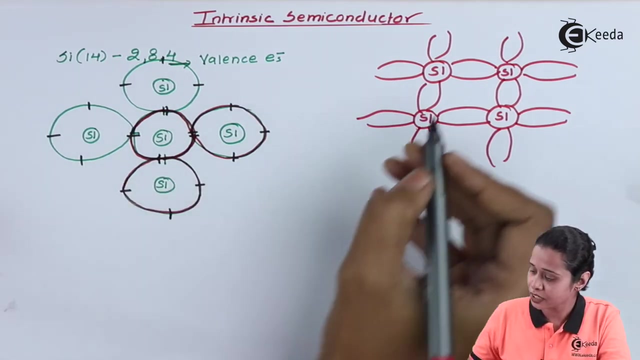 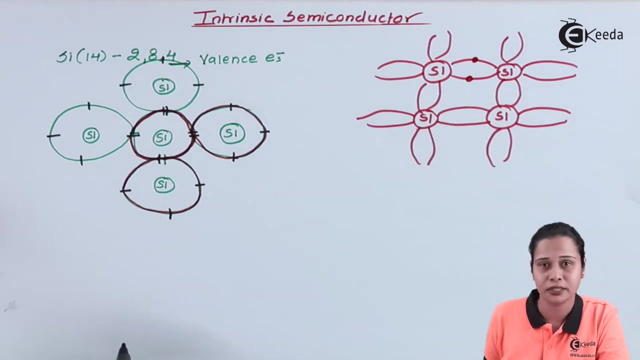 for this diagram. So in this way we can draw the silicon solid. So here we can say: this is the electron belonging to this silicon, and the another electron is belonging to this silicon. So in this way there is a covalent bonding between silicon-silicon atom. 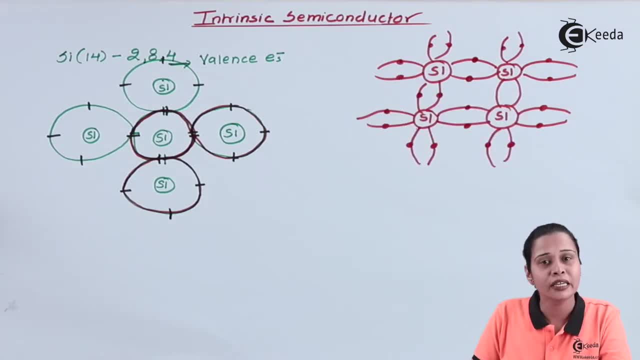 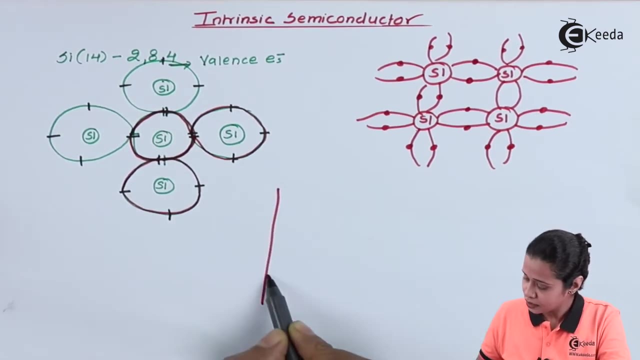 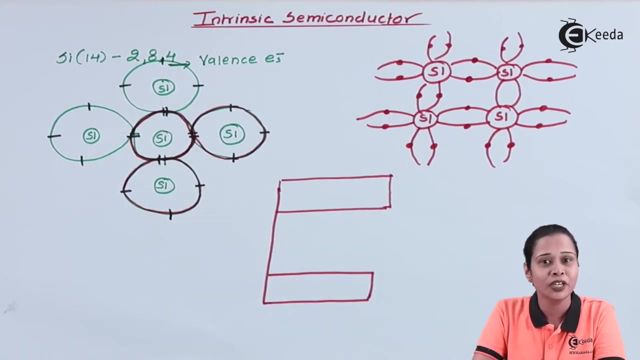 Let us understand the concept of band theory in case of the intrinsic semiconductor. Now we know, in case of intrinsic semiconductor we have covalent as well as conduction band also. So we will see, this is a covalent bond. So in case of semiconductor, we know there are two. 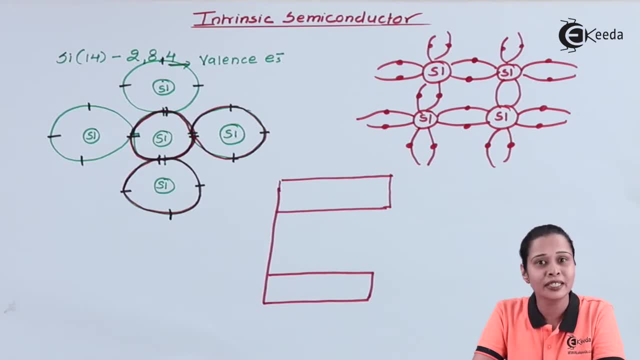 bands, conduction band and the valence band. So let us understand the concept on the basis of band theory. So in case of intrinsic semiconductor, we will consider: here we have a valence band and the above we have conduction band. 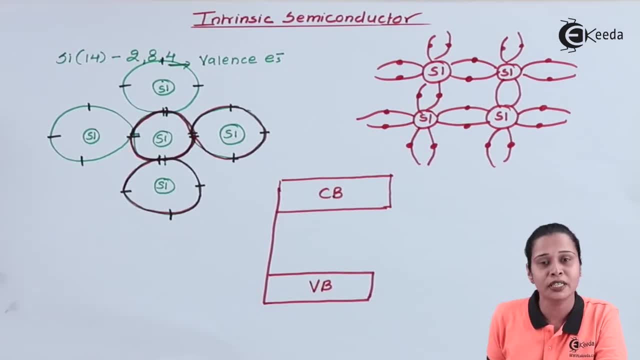 Initially just say: suppose temperature is less than, or we can say it is less than room temperature. In that case what happens? All the electrons are tightly bound in the covalent bonding Means. there is no free electron at very low temperature. So we can say: in that case, 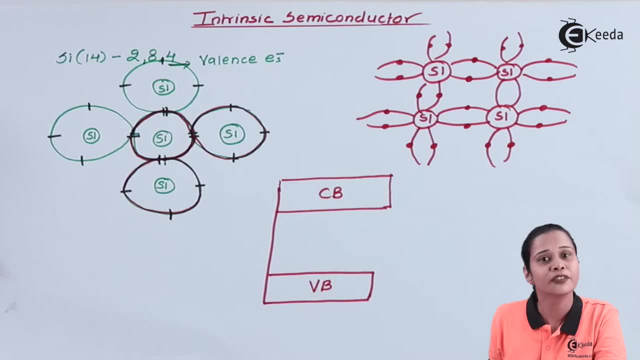 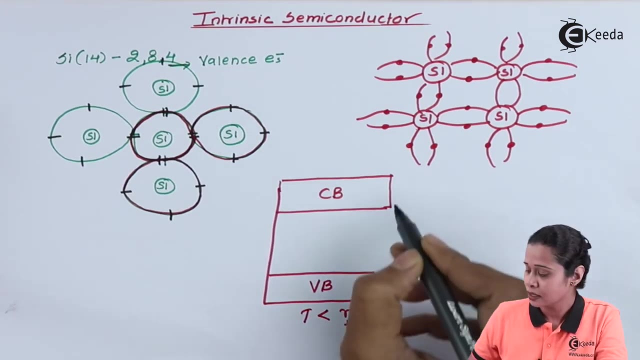 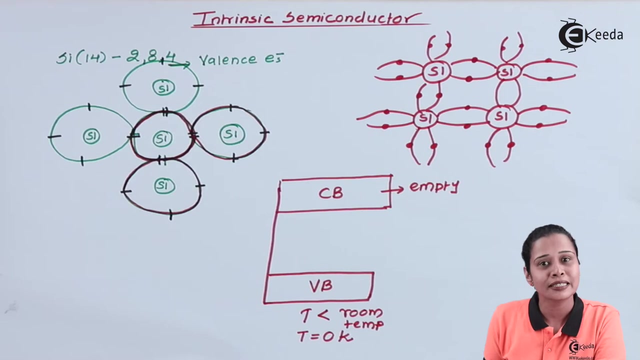 conduction band is empty and valence band is fulfilled. So let us consider the example T. It is very less than room temperature. In that case the conduction band is empty If the temperature of material is less than room temperature. 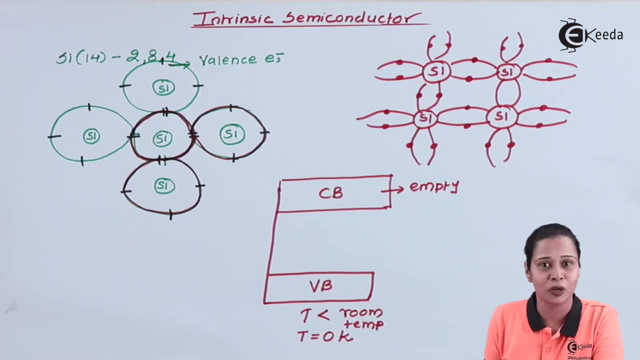 then all the electrons are tightly bound in the covalent bonding, So there is no free electron. So in that case we can say conduction band is empty and valence band is fully filled. Now let us consider another case, That is, temperature is greater than approximately. 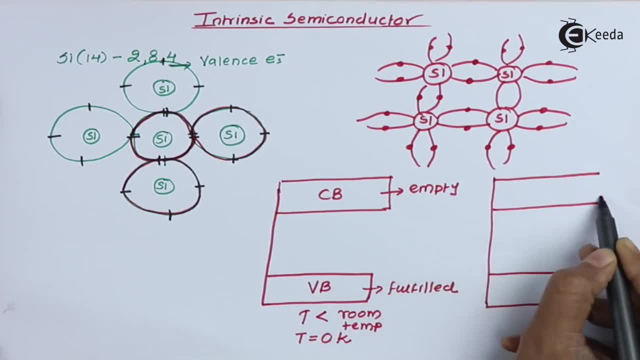 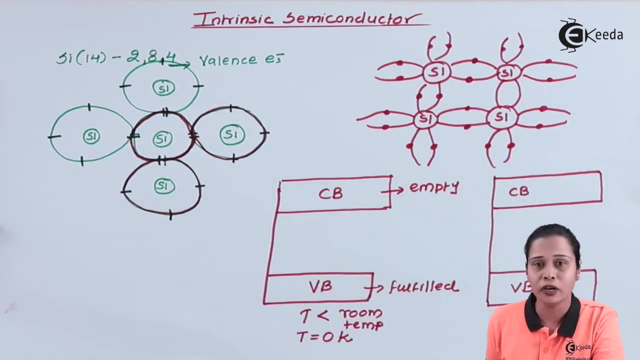 equal to room temperature. Now, when the temperature of material is greater than room temperature, in that case the covalent bond will break. After breaking off this covalent bond, just example: suppose there is one covalent bond which is breaking. Now there is a free electron. 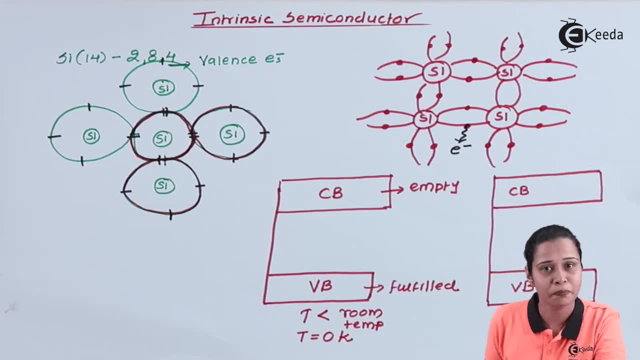 This electron now available for the conduction. but after breaking of covalent bond there is a formation of hole in the covalent bond. So we can say there is a empty space in the covalent bond, or we can say it is a deficiency of electron in the covalent bond and that deficiency 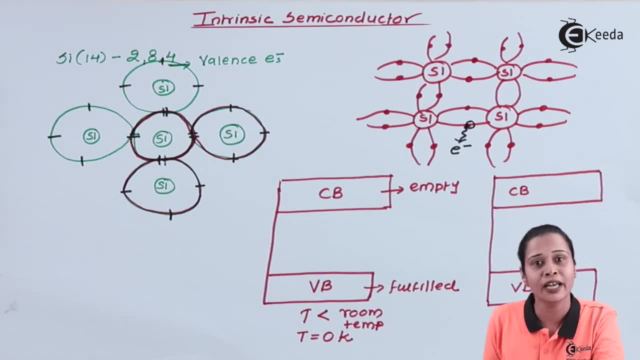 or absence of electron in the covalent bond, called as holes. Now we know this. all bonding are present in the valence band and the free electron. this is available for the conduction, So we can say this is conduction electron. 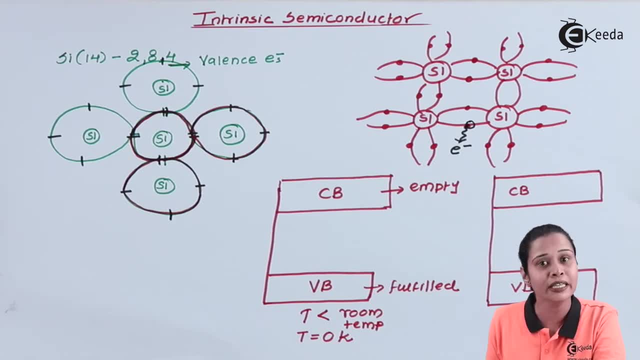 So we have to show the position of this conduction. electron in the conduction band. So we can say at temperature which is greater than room temperature there is a electron in the covalent bond So we can say this is available for the conduction. So we have to show.